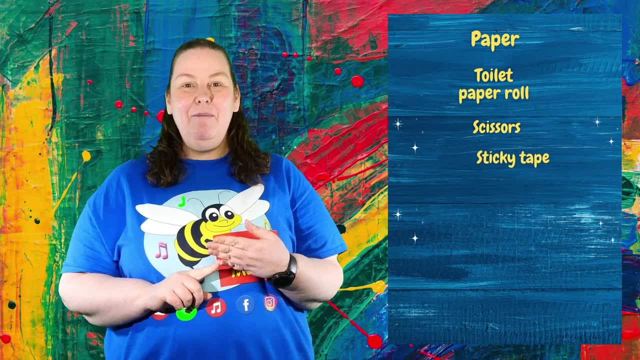 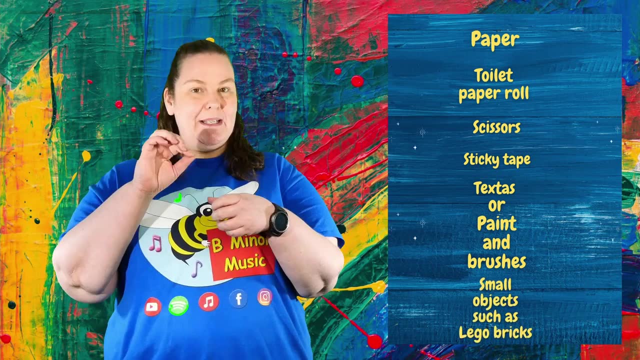 in half. We'll need some scissors, some sticky tape, and we'll also need some textures or some paints so that we can decorate it, and we need something small that we can pop inside to make the shaking sound. So you might like to find some pebbles or some tan bark around the garden or inside your 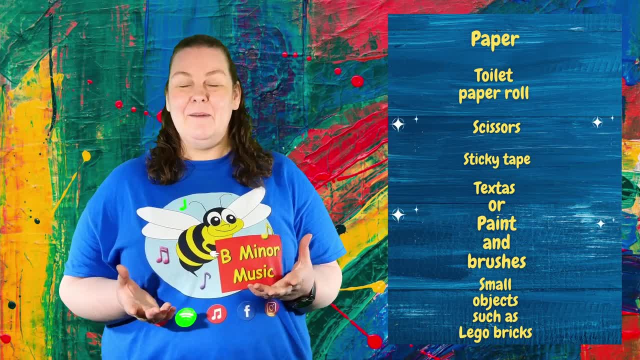 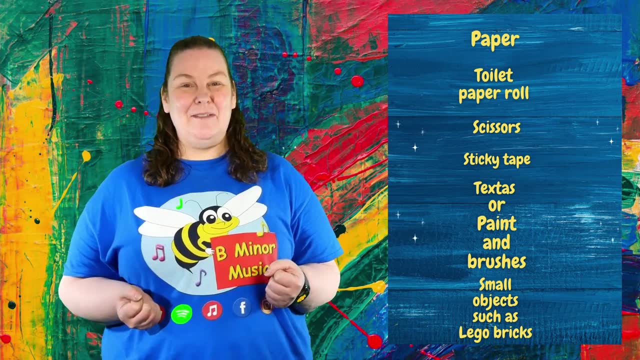 house. You might have some small toys that you can use- I like to use lego pieces- or, if you don't have any of those, have a look in your pantry and you might have some uncooked rice or some uncooked lentils that you can use All right now. before you go off and get those, pause the video. grab all. 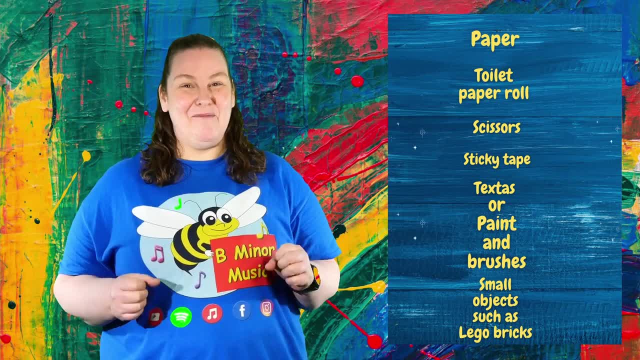 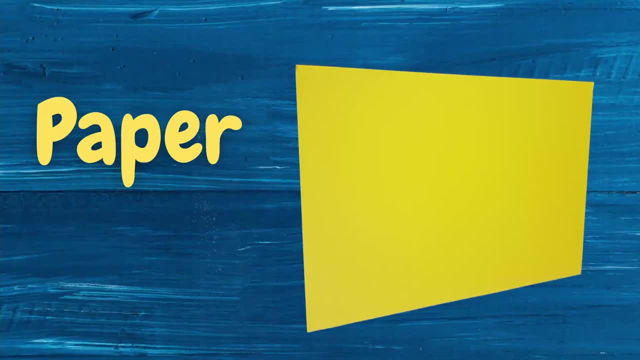 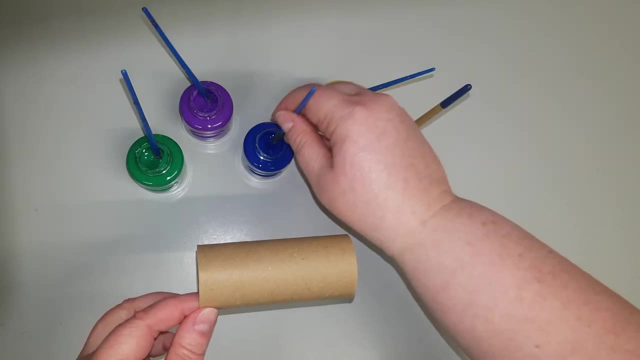 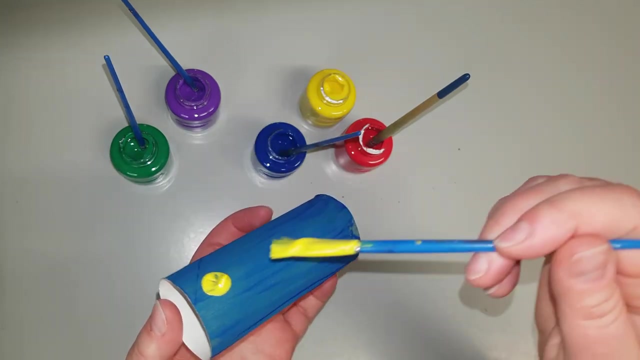 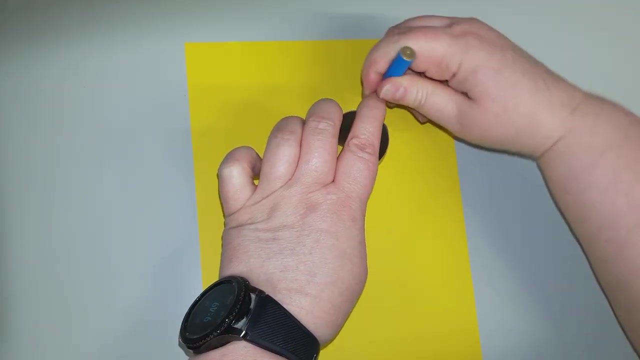 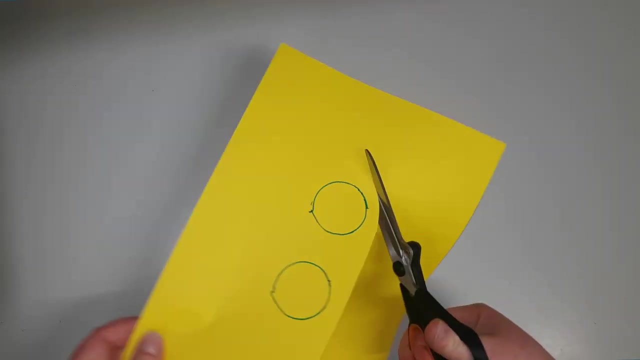 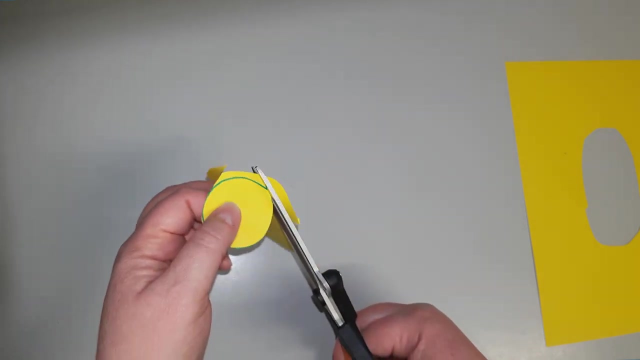 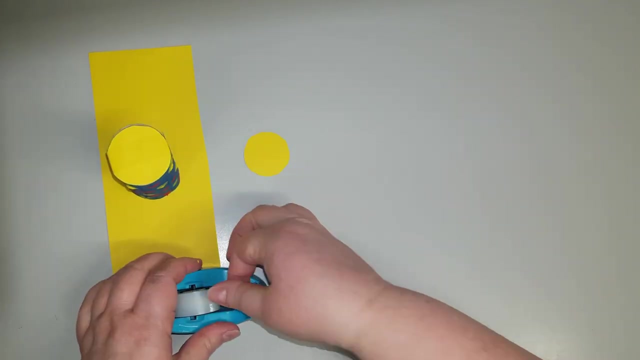 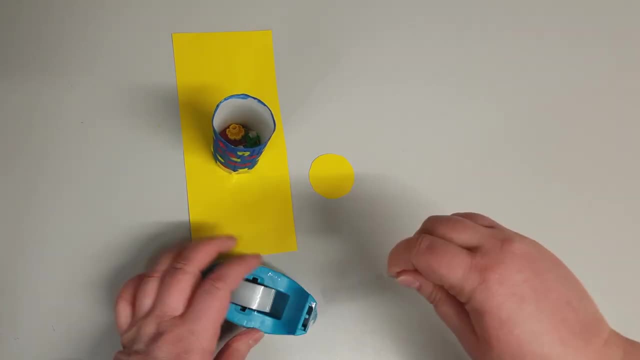 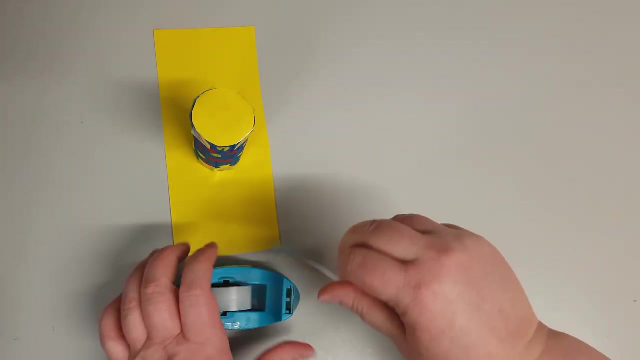 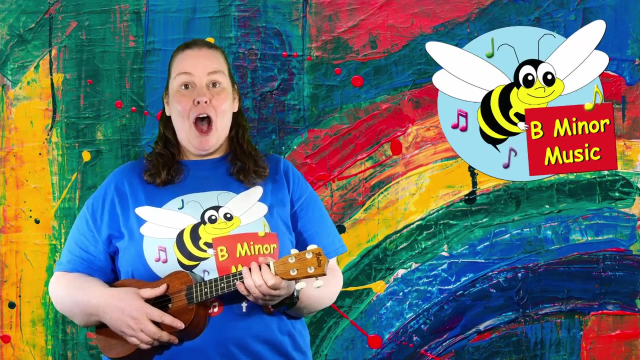 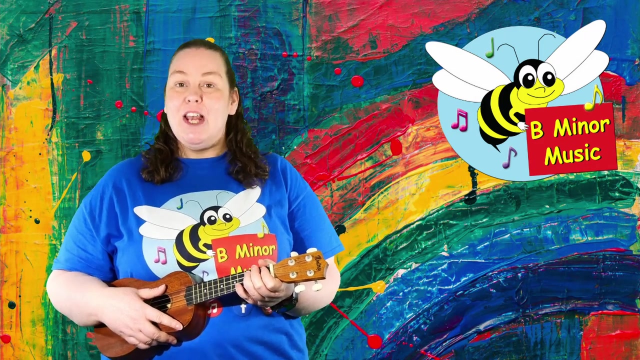 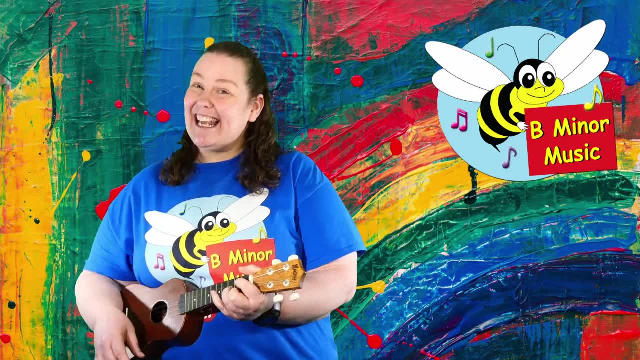 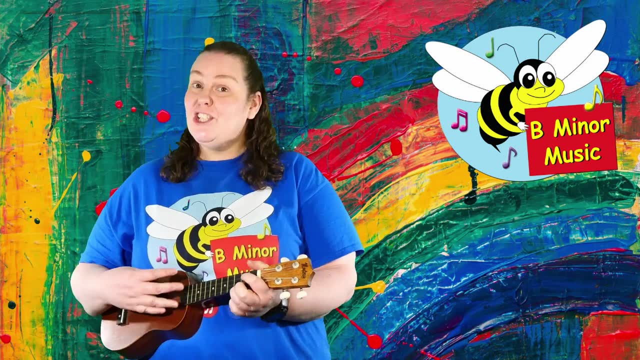 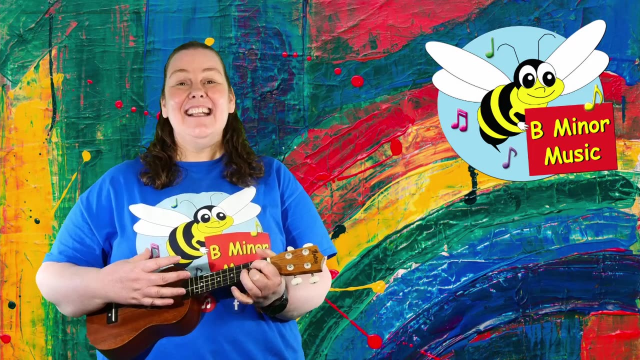 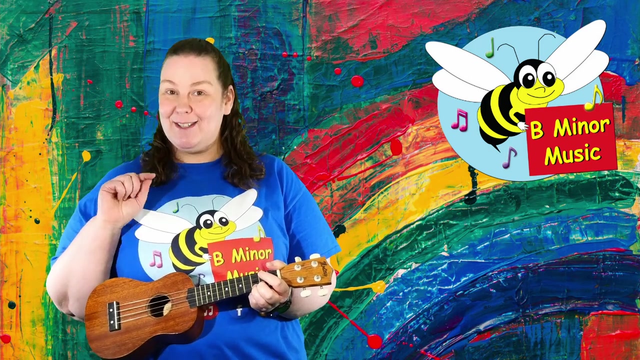 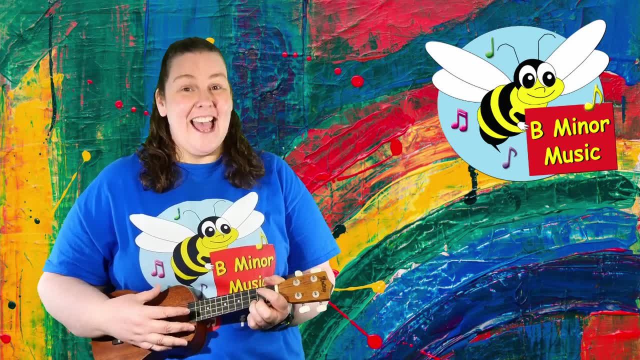 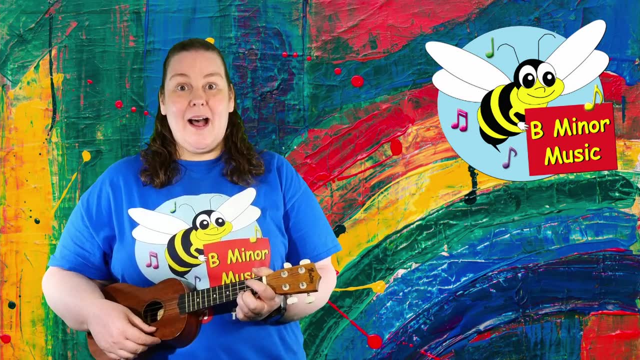 shaking slowly, shaking. everybody's shaking really slow, but it's so much more fun to go faster. Everybody shake, shake, shake, everybody shake just like us. everybody shake, shake, shake, everybody shake, just like us. 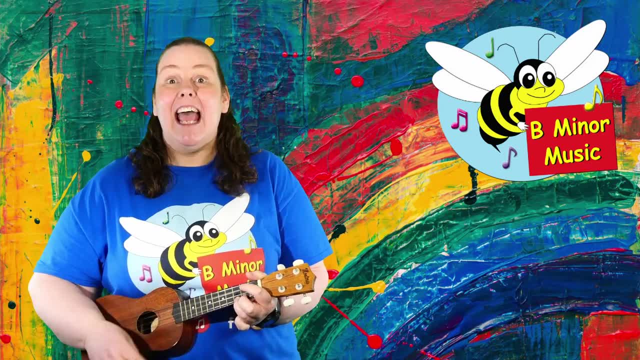 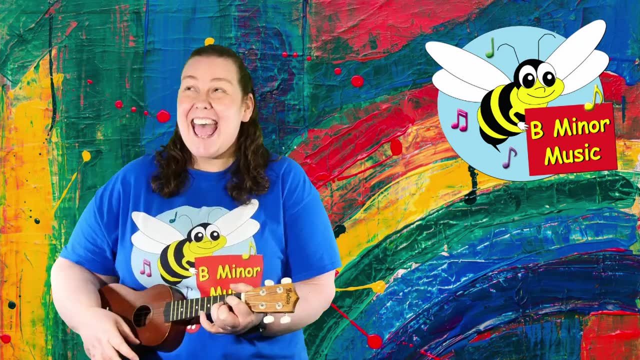 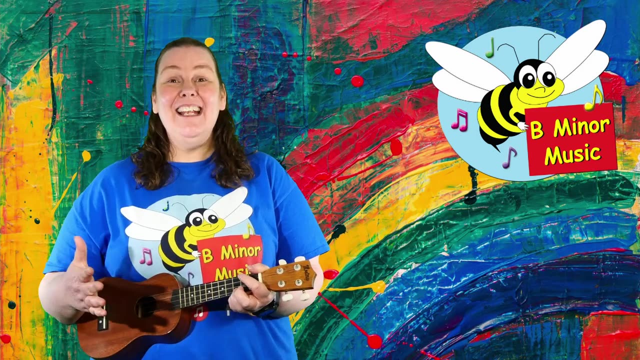 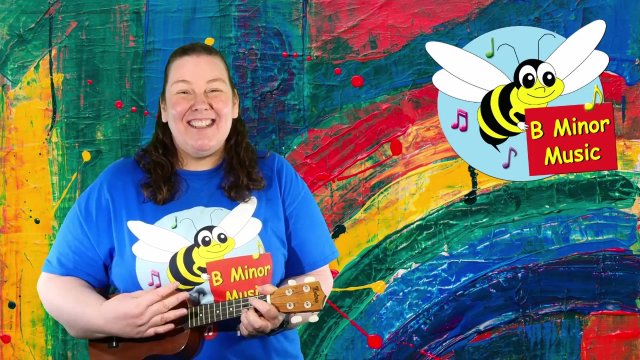 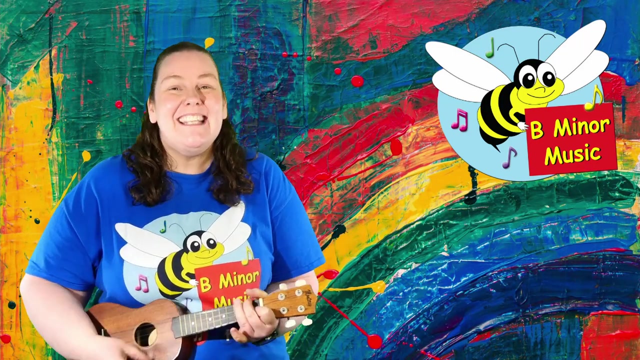 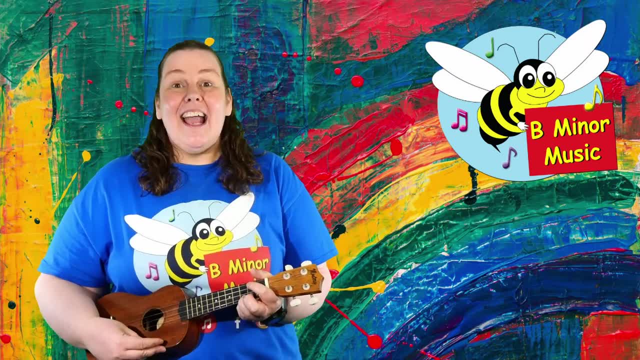 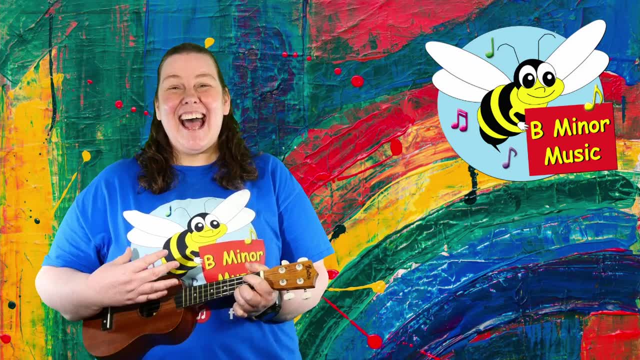 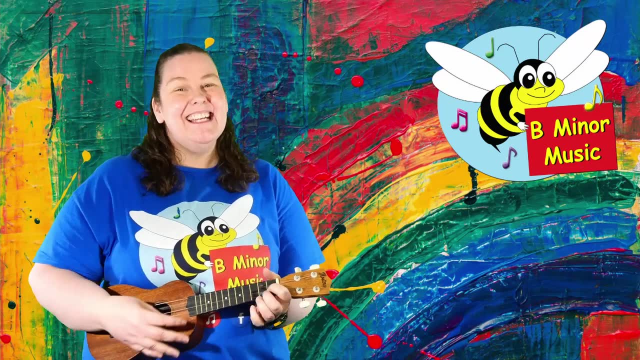 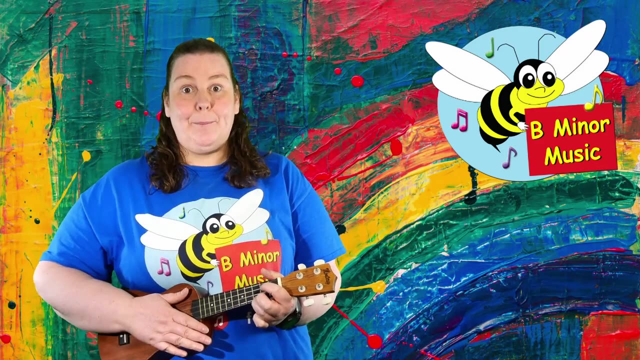 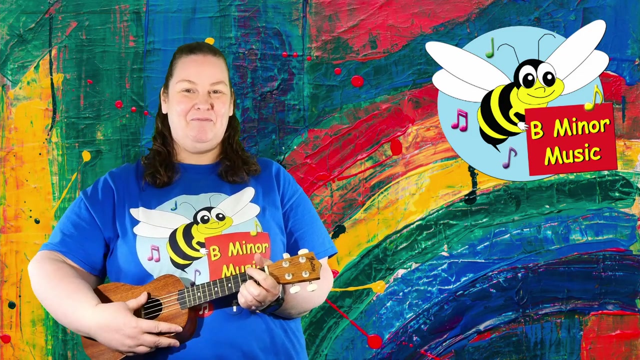